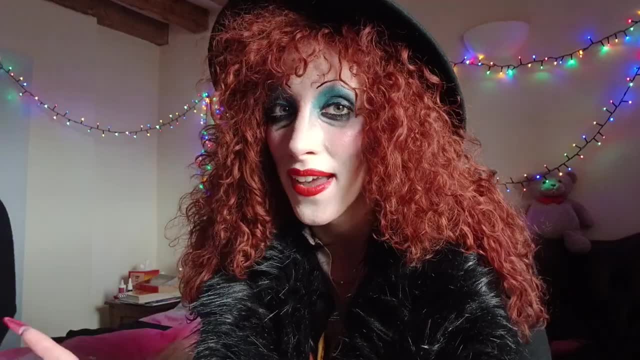 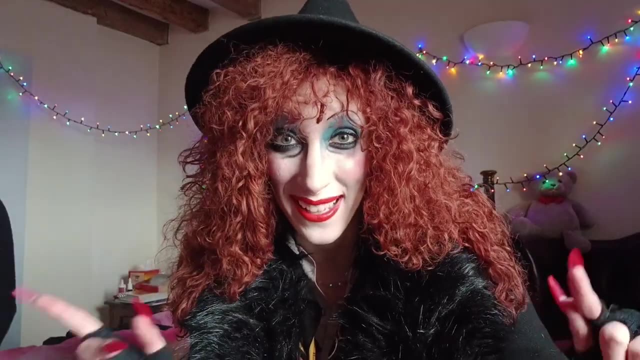 putting any dye on is I'm going to anti-dandruff the hell out of it. I'm going to go and scrub my hair with anti-dandruff shampoo, then just blast it dry and comb through it. then we'll start putting the dye on, okay, So I just did what someone with curly hair should never do and just rub my hair. 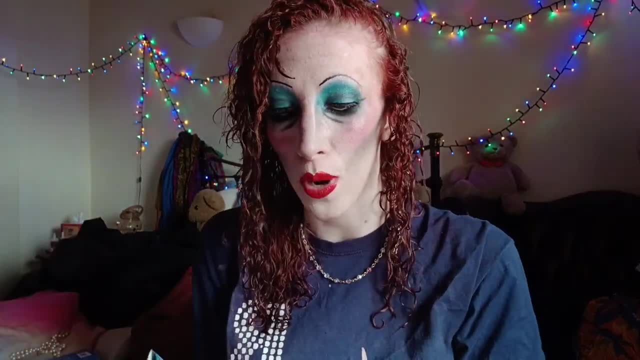 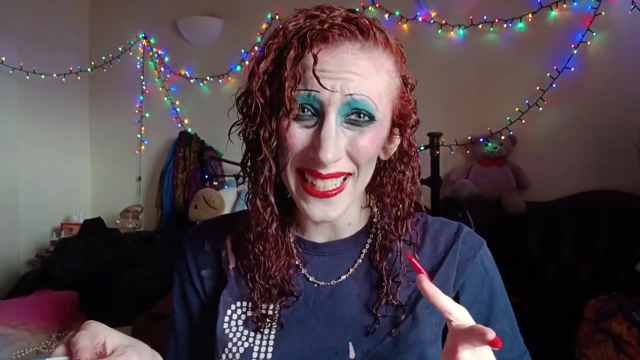 with a towel, but coincidentally, I'm going to dye my hair again. I'm going to dye my hair again. I just came in to read the instructions- Not that I ever read instructions, but I haven't used this one in a while- and it's the consistency slightly different to normal hair dye for some. 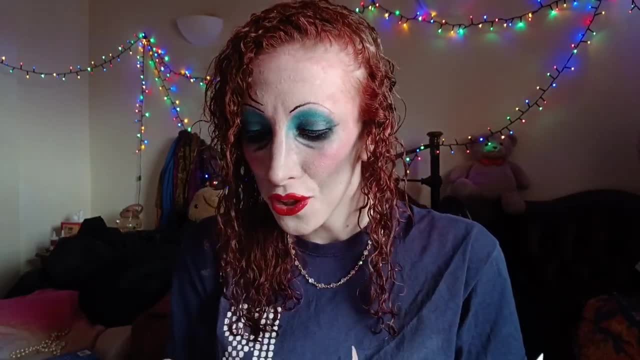 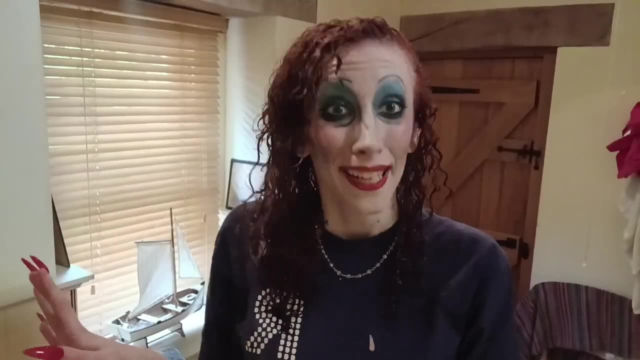 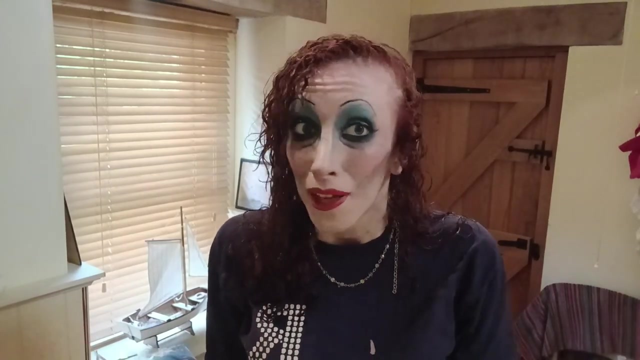 fucking reason. so I thought I'd read the instructions and it actually says you should put it on damp towel, dried hair. so good fucking job, I washed it, isn't it? Hello, and welcome to my bathroom. I apologise for the lighting and the angle, because this is all we've done. 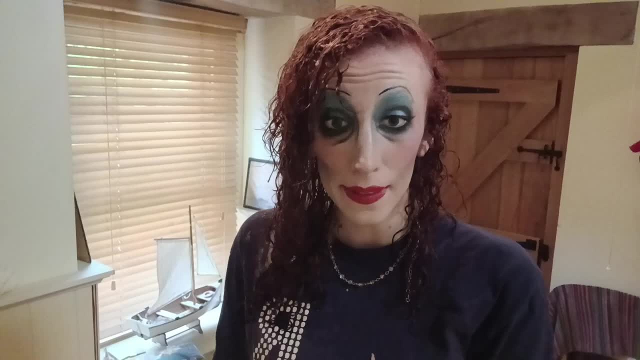 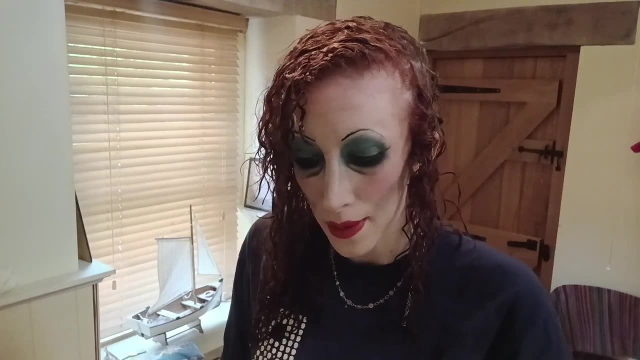 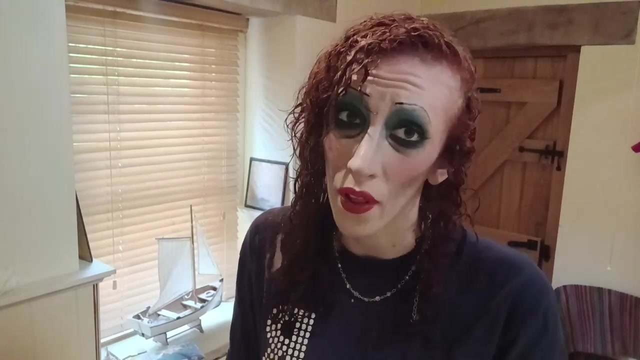 We've got so fucking deal with it. First things fucking. first, the gloves they give you in boxes of hair dye are always absolute crap. so I just went to the local pound shop. You know the kind of pound shops you find on the corners that definitely sell drugs behind the counter. one of 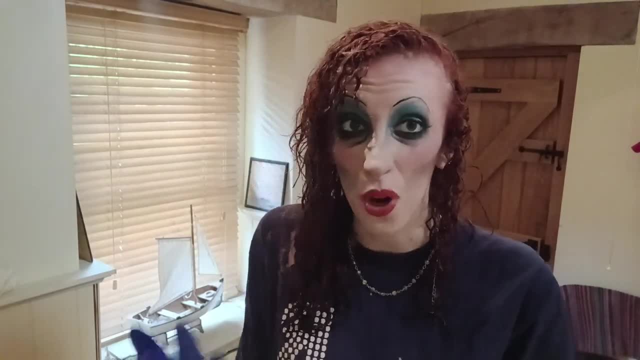 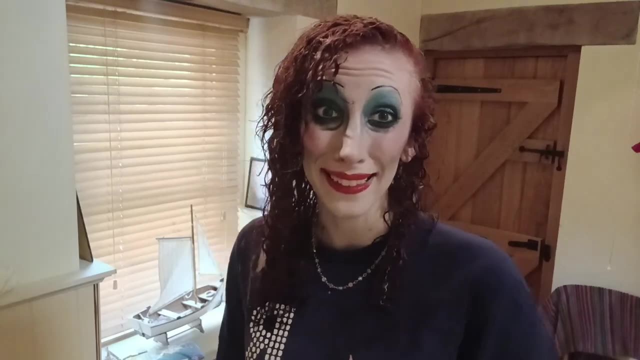 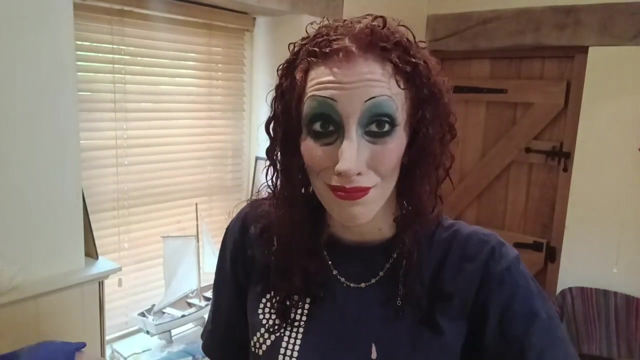 those, and I've got so many boxes of these kind of gloves. Surprisingly, they do fit over my fucking talons, so that's a great start. Also, I've got no idea what I'm going to do with this. I'm going to dry my hair while the fuck it's gone into this kind of comb over. Not that it matters, it's going. 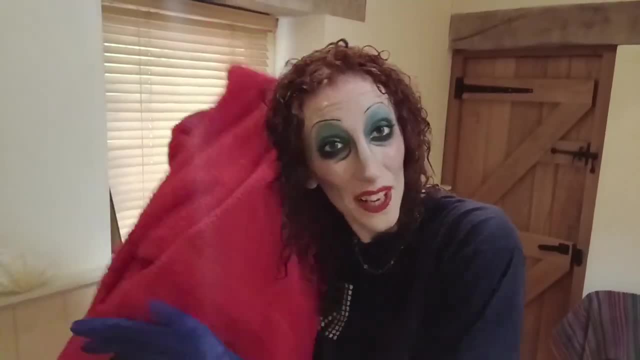 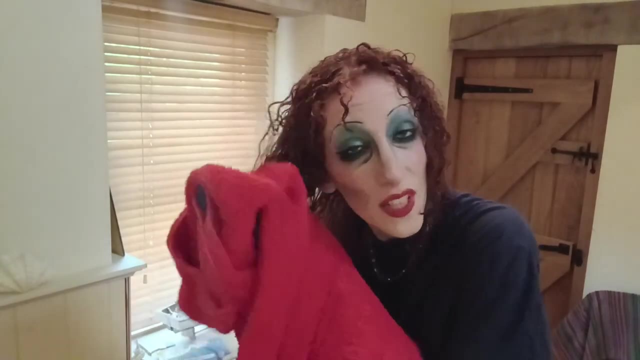 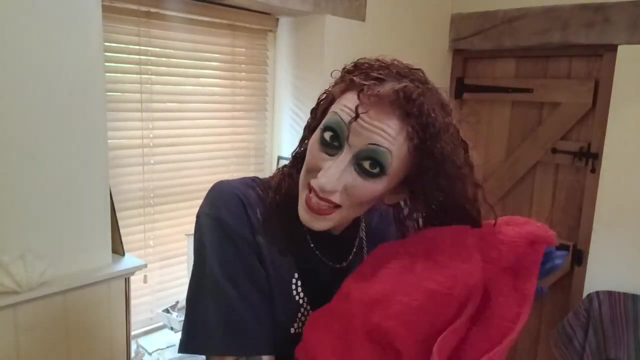 to be dyed soon- in a minute anyway- but I do feel like I should dry it some more. but this feels absolutely sacrilegious to do, because this is one thing you never should do with curly hair, unless you want what I'm going to call instant magenta hair. This just gives you frizzy hair. 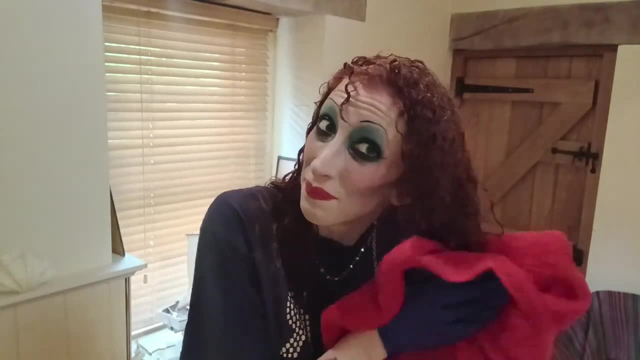 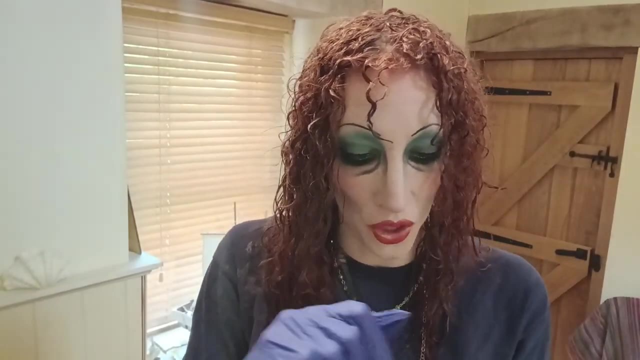 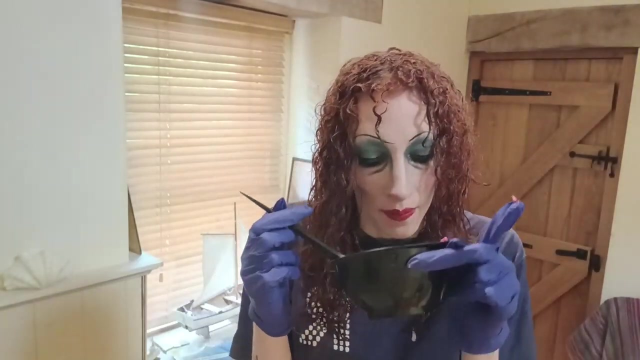 for days like you can literally see it coming. but it doesn't matter what happens to the curls anyway, because it's getting dyed Now I'd honestly just buy. has anyone ever used the live pink dye? Because I would honestly buy a perfume of this stuff. 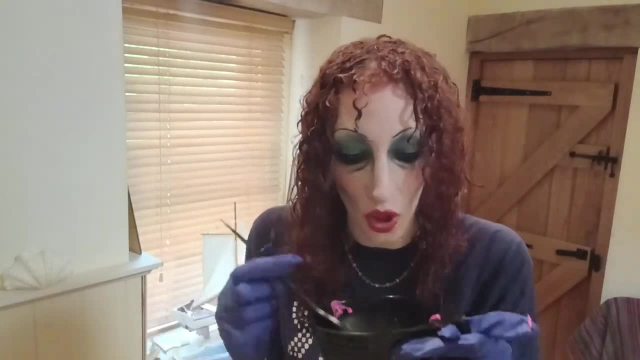 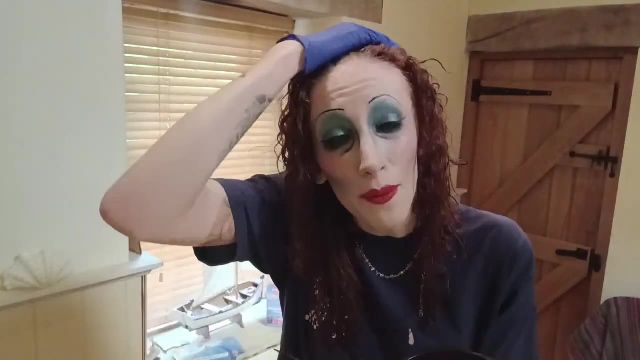 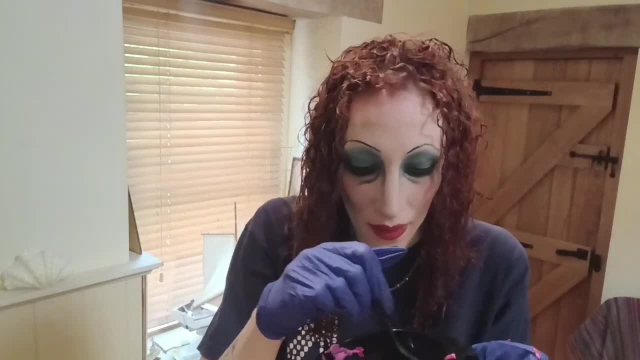 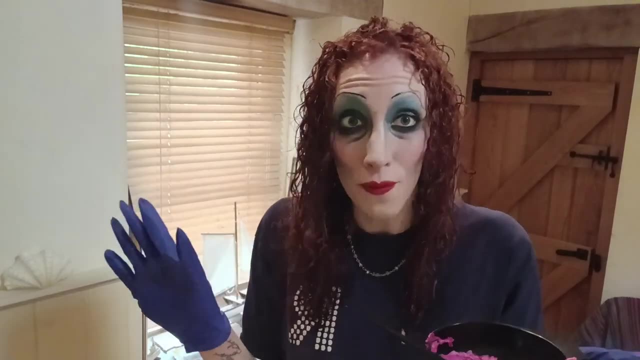 know, I don't know, I don't know- I'm not even going to say that- but if you're going to dye your hair, just buy this and smell it and you won't regret it. Cause that is sexy, that If you don't even want to dye your hair, if you don't want to dye your hair, just buy this and smell it. you won't regret it. It's amazing. 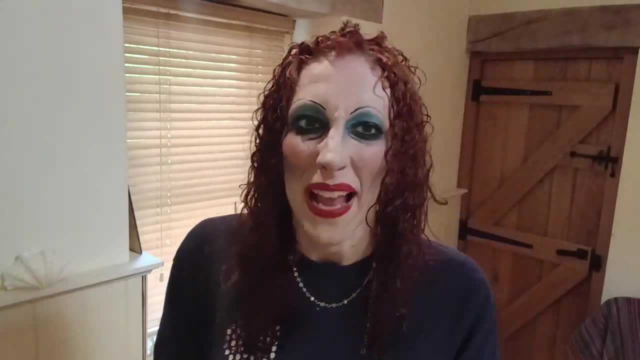 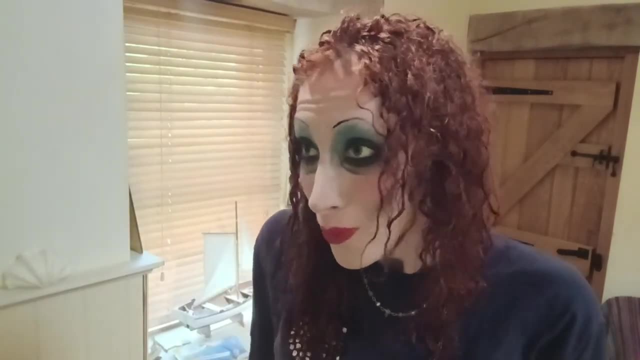 If you don't even want to dye your hair, just buy this and smell it. you won't regret it. It's amazing. Now I'd like to apologise for the angles, because the camera is here. there is my mirror, So you're going to get some interesting shots, but I do know the actual way you're meant to dye your hair, because I've been doing this for about 3-4 days. 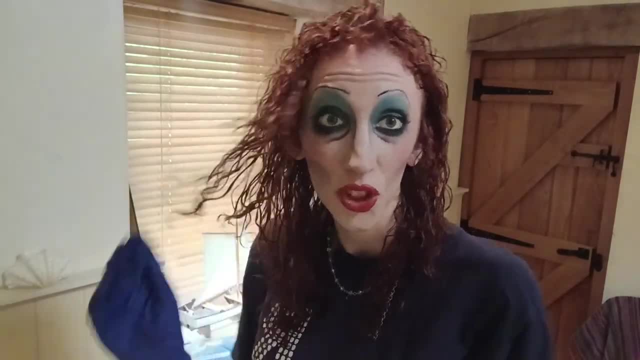 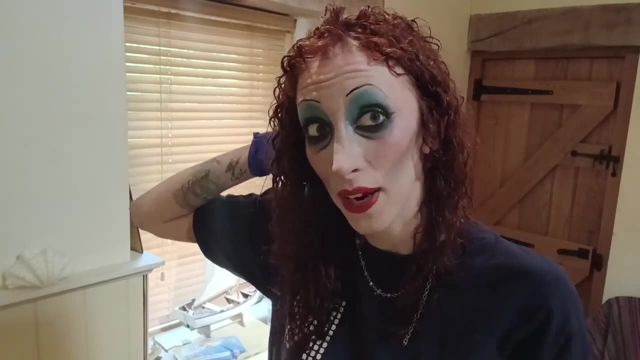 um, my best friend is a qualified hairdresser and she taught me how you actually, how they actually do it in salons, like the way they do it. but what actually does tend to happen is i start off with great intentions, you know, i put it on the hairline, and then i put it on the parting, and then i get. 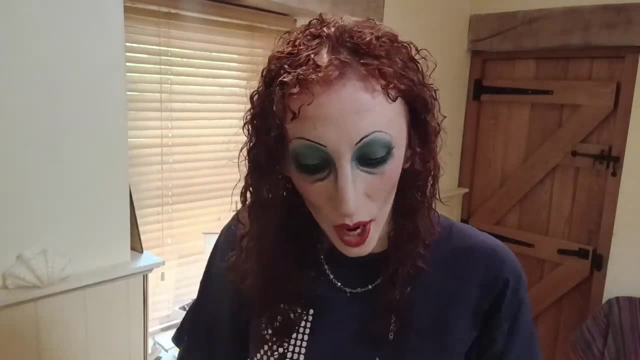 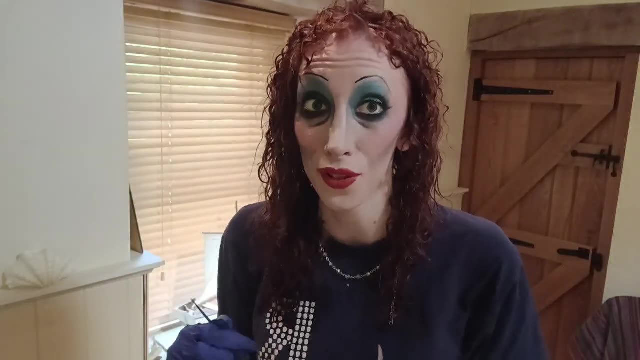 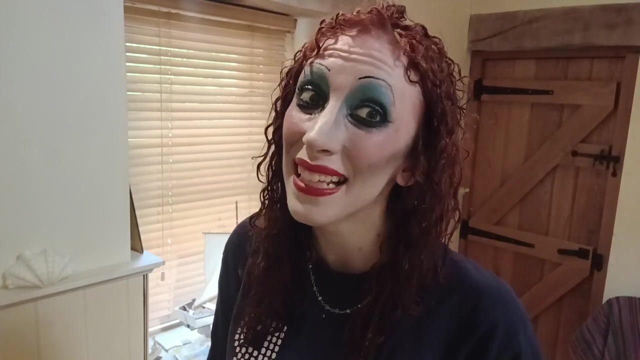 bored. then i get bored and i just kind of start slapping it on. but yeah, i have two boxes in here, which i'm hoping is enough. if not, we're going to use the good old method. i'll put some conditioner in there and pray, which worked out for me last time i dyed my hair. so, um, let's get this shit. 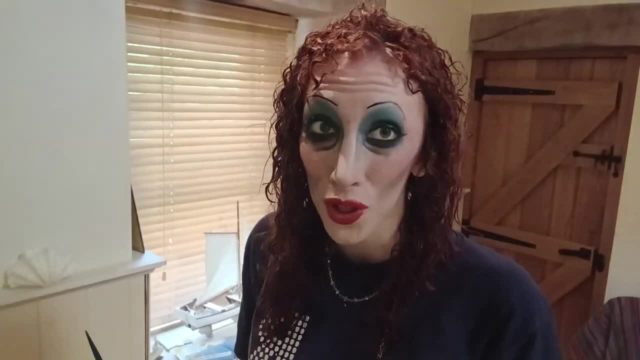 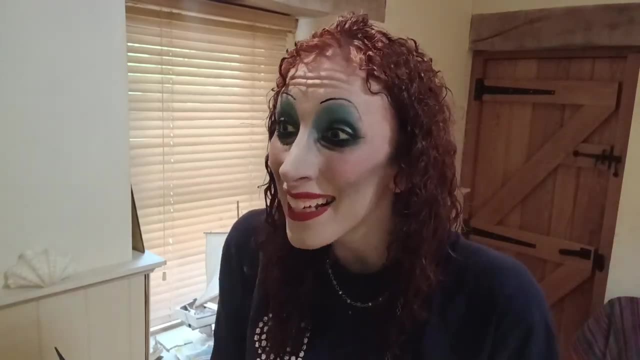 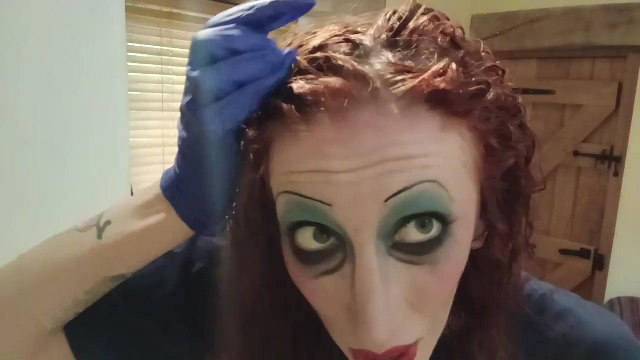 show on the road, shall we so in um just pressing um record on my camera, i accidentally got hair dye on my phone screen. let's hope that doesn't fuck with the um phone too much. i don't know if you can see in this lighting, but um, i do have some very, very slight roots. yeah, you can see them there. 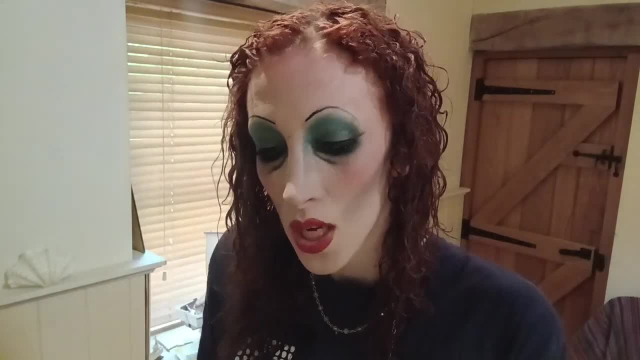 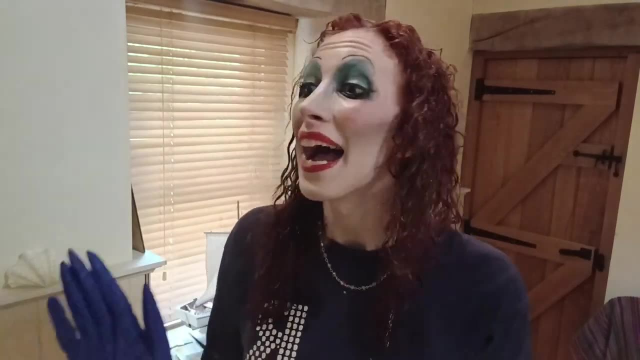 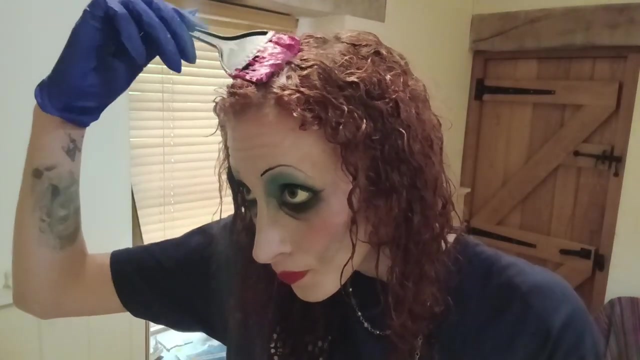 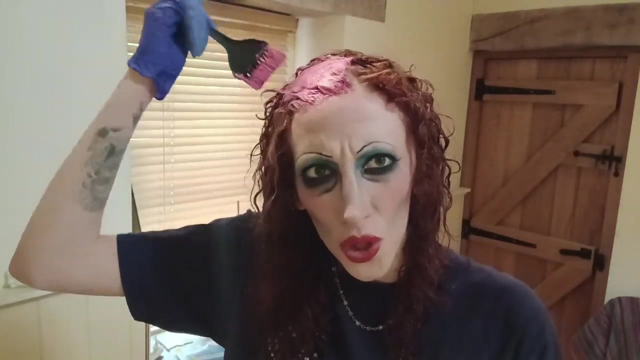 because, um, i'm a natural blonde, you know, this is the moment, you know, when you dye your hair and you, just before you start and you go, i could turn back now. i could turn back and nothing would happen, but, um, i'm an impulsive mess, so we just slap it on. you know, i really really am too. i don't know if the word's lazy, i don't. 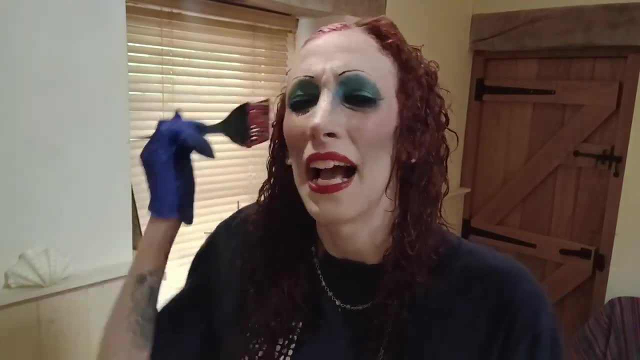 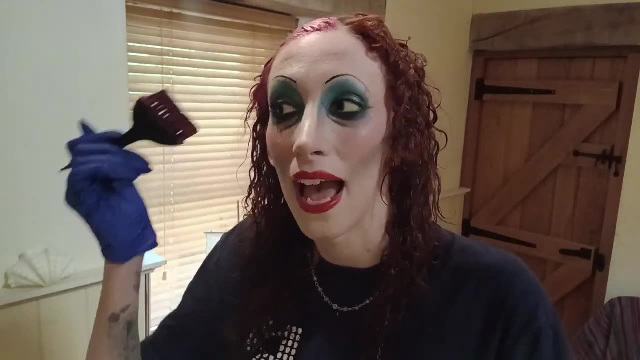 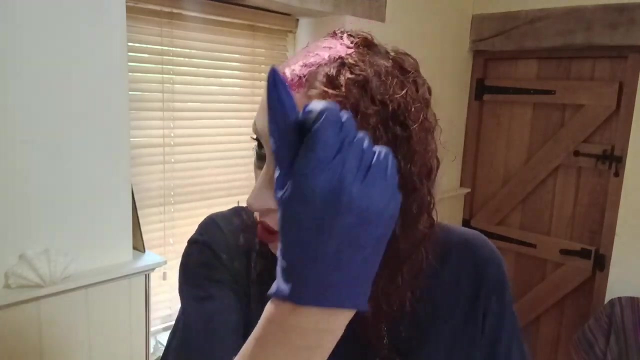 think it's lazy, i think i'm just too um. i don't think the word's impulsive either. i don't know. i don't have the patience to um dye the hair, my hair- the way you're meant to, and if you actually comb through my hair, like right now, you'll see a lot of spots where i missed. 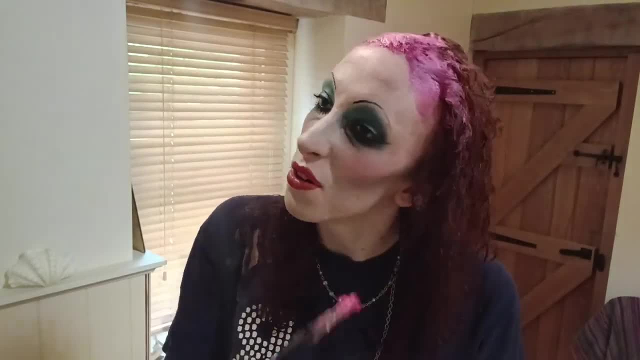 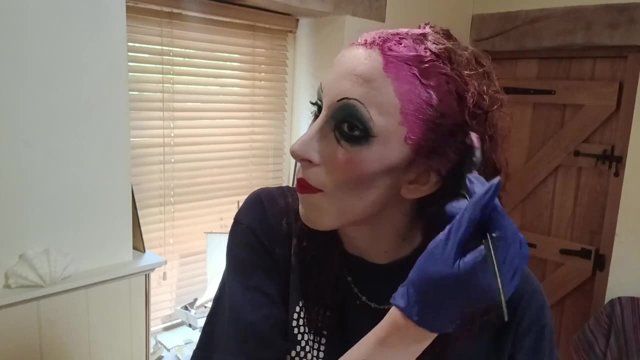 it with the ginger dye and there's just a load of blonde roots and i don't really care, to be honest, like that's on the inside of my hair. so as long as the front, as long as it looks okay from like the front, what's going on in the rest of my hair or the back, none of my business, um. 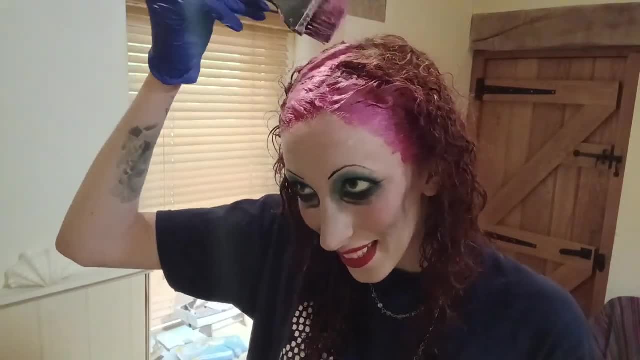 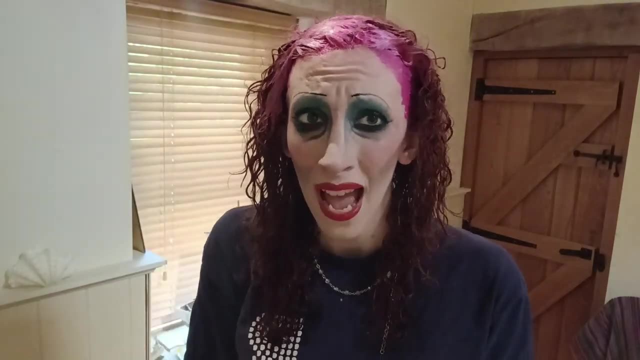 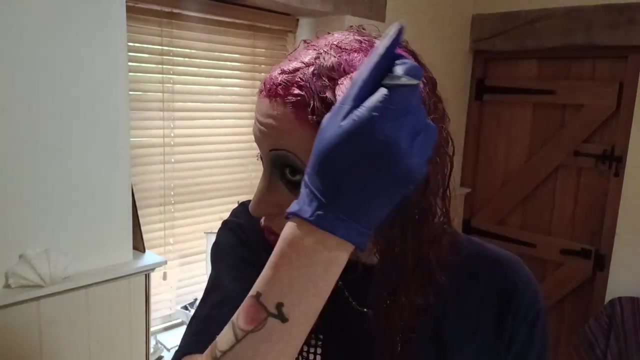 i can tell already that this is going to be such a look because, while i'm slapping this on, let me tell you the story of my pink hair. so i dyed it when i was 18. essentially, what happened is i did my a levels, i did my level exams. then, literally the day after i finished my last a level, i went. 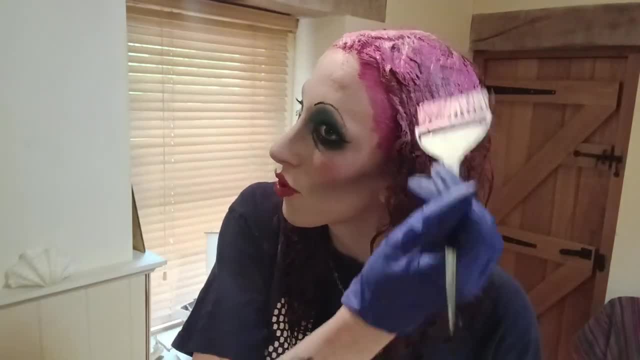 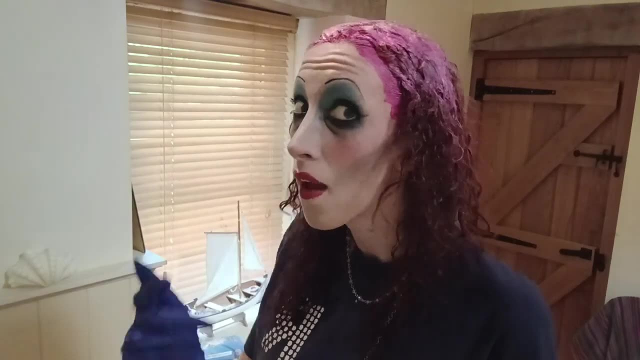 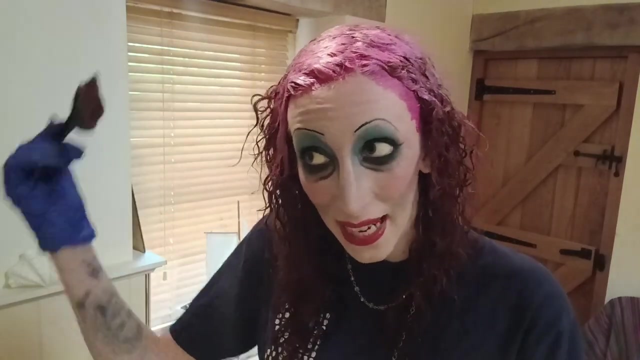 on a cruise for two weeks and then, two days after i went on that cruise, i um got my nose job. fun fact one day- my nose job because this is fake, but anyway, while i was on said cruise for two weeks, i wanted to dye my hair pink. i'd dyed my hair ginger before. i had ginger hair then. 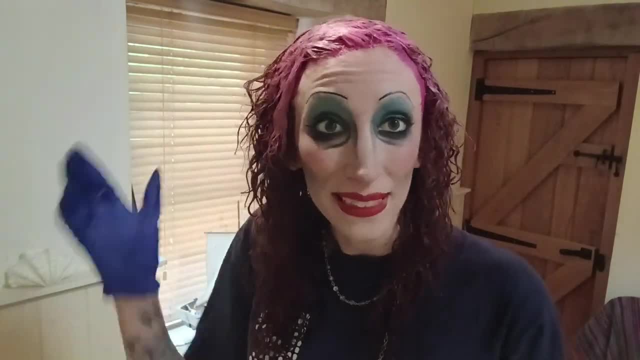 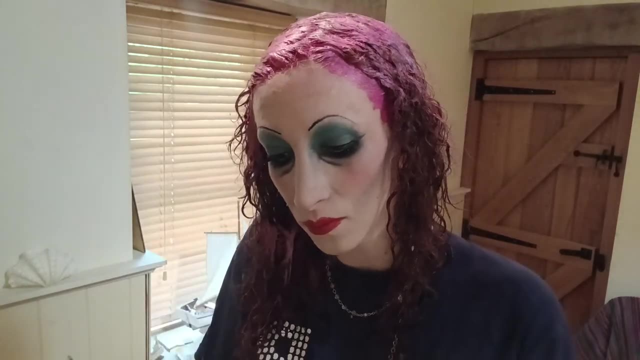 because, as i said, i've had ginger hair for a long time but i wanted to dye it pink. i've never done this is this would be the first time i did a colour that wasn't um natural. but i wasn't allowed down my hair as a kid for the longest time. my mom dad just said: no, you've got to keep it, your natural. 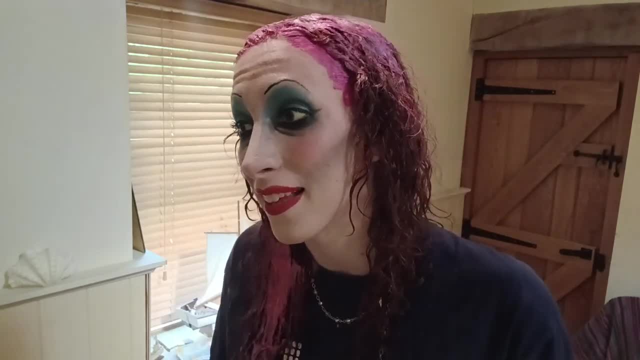 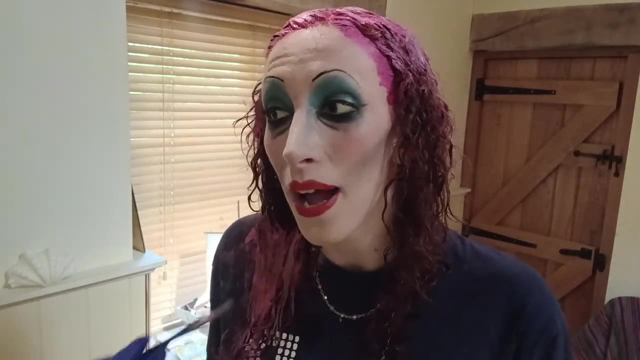 color and when i was 16, i was allowed to dye it ginger. but obviously i was 18 at this point. i could do whatever the fuck i wanted, and i wanted to dye my hair while i was on the cruise. so i went to the in cruise salon- which is a thing they do on royal caribbean- and, um, they did a test. 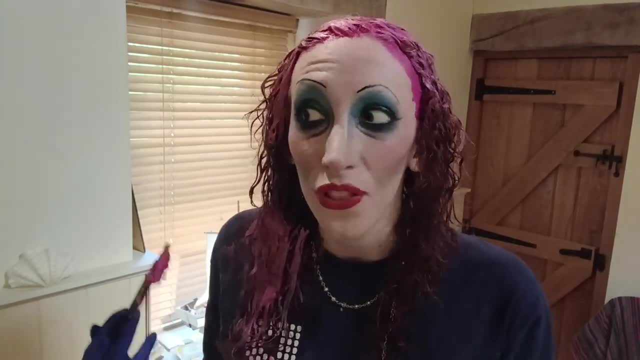 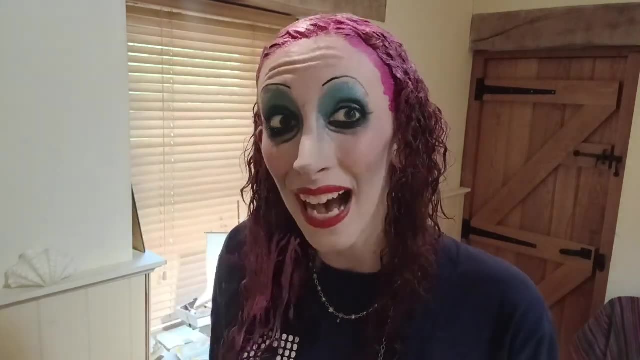 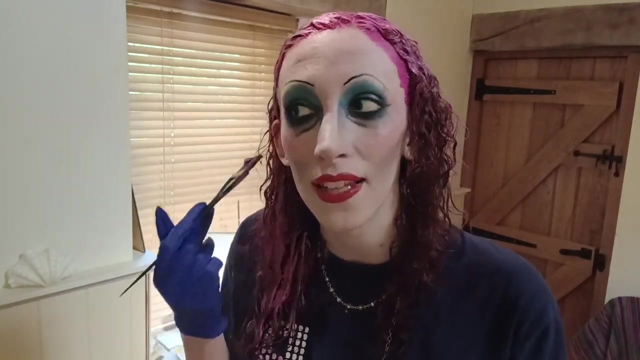 and it was like the most amazing bright pink color ever. but the price they wanted from me was a lot of fucking money and i didn't get my first job until i was 21 and after i graduated uni. so, um, i didn't get that done and, honestly, i kept looking at the strand, like every time i 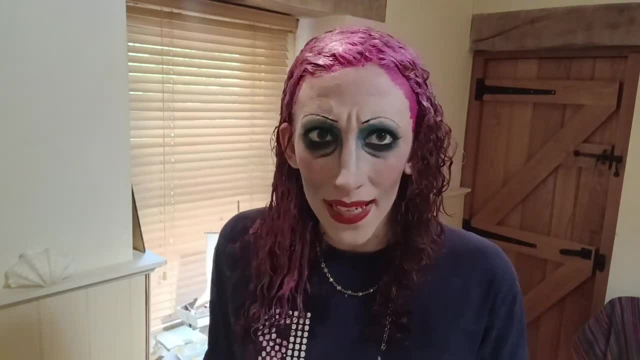 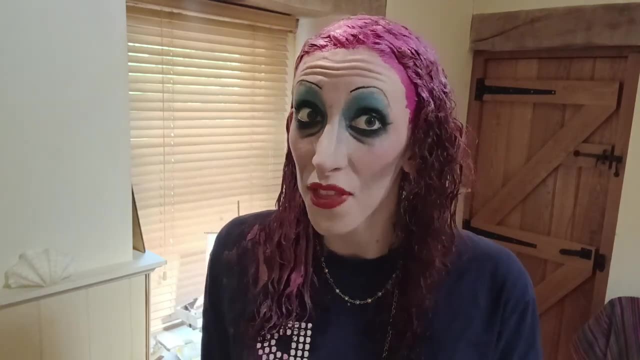 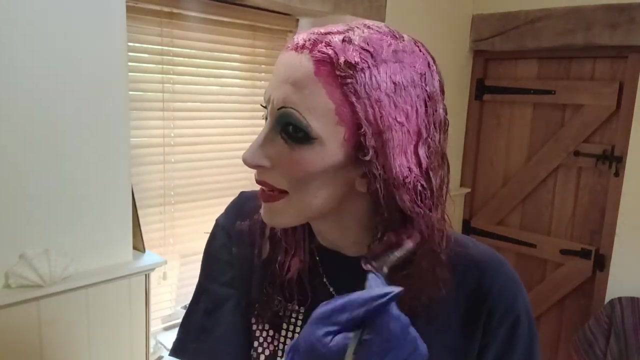 washed my hair on this cruise. i looked at the strand. they died and, not even kidding, the strand went um, blonde, like the color came out the strand really really fast, like it was ridiculous how fast the color faded. so it's probably a good job. i didn't do it then and a couple of times when i 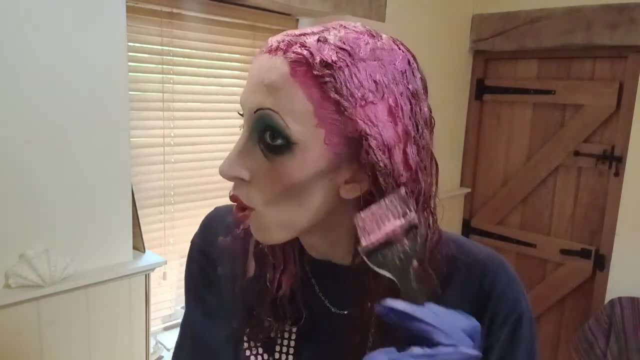 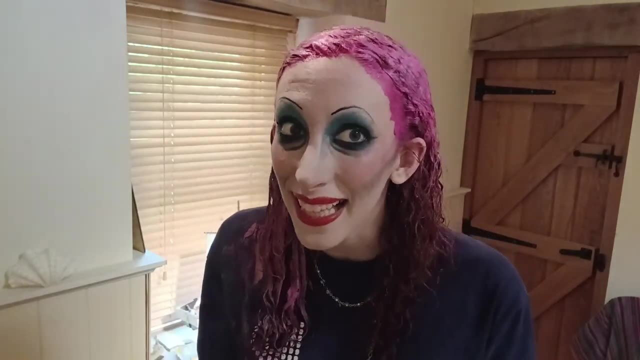 got off in the port. i went to salons in the port trying to ask them how much it cost to lighten my hair. but the thing is, the place i asked was in italy. obviously the ladies in the salon, funnily enough, they spoke italian. they. 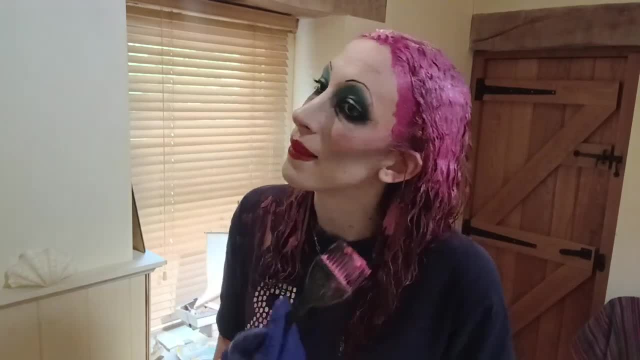 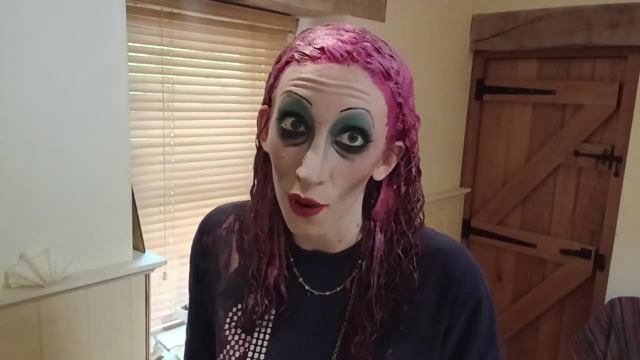 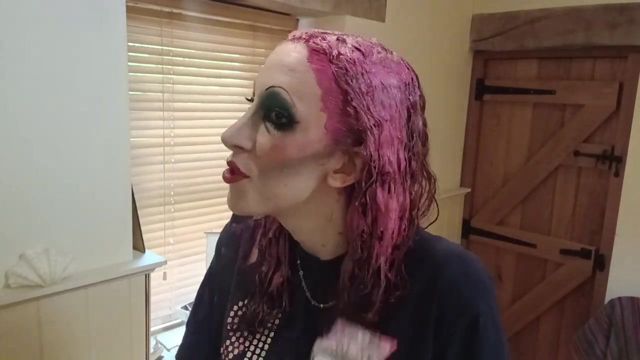 didn't speak english, but i know that i can't have my hair bleached because it's too um like damaged. so i was trying to say: can you dye my hair pink before the boat sets off and leaves me behind, and not use bleach? but obviously it wasn't really working out because i was using- we were both using. 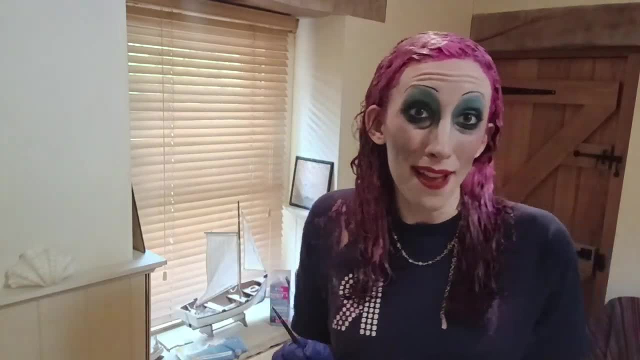 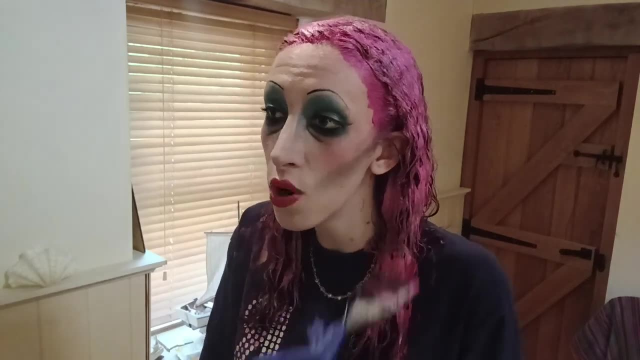 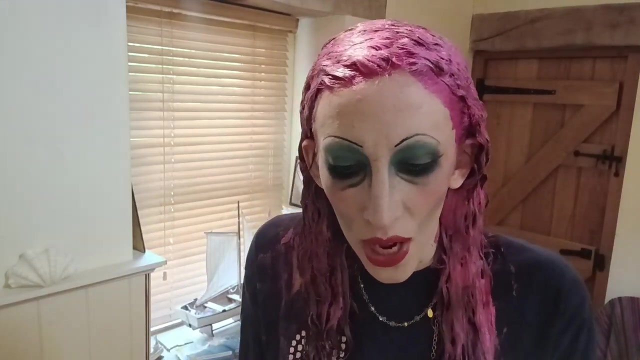 bleach trying to talk to each other and i was like this is a bad idea. so i never got it done on that cruise. long story, fucking short. but um, two days later got back, got back home and had my nose job waiting for that to settle down. then i dyed it pink, but i used um- was it manic color or something? 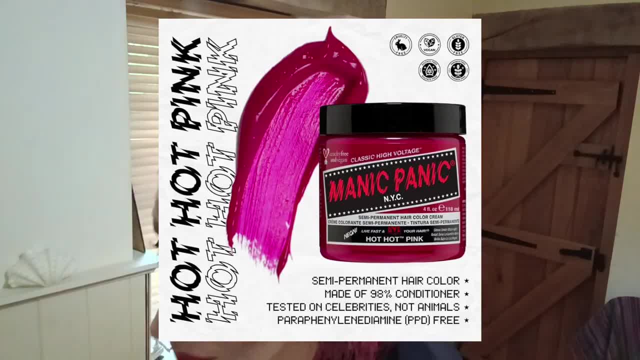 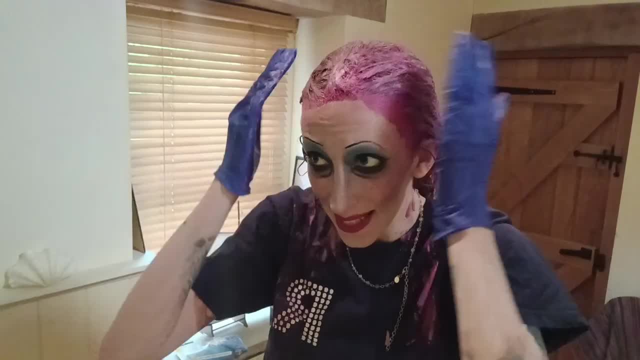 i think it's called some. i might be getting that wrong, but it's called the brand, something like manic color. it's quite an iconic brand and i used that and i got it from like a shop that does like piercings and stuff. i got it from one of those. 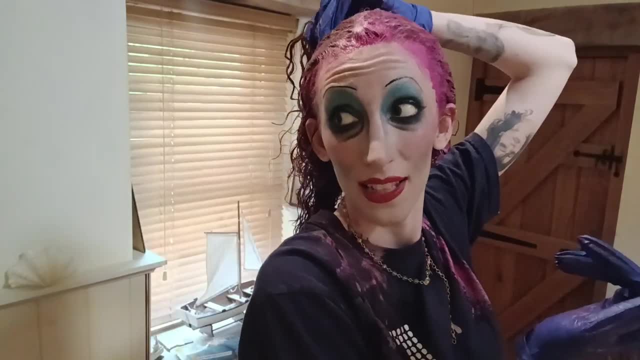 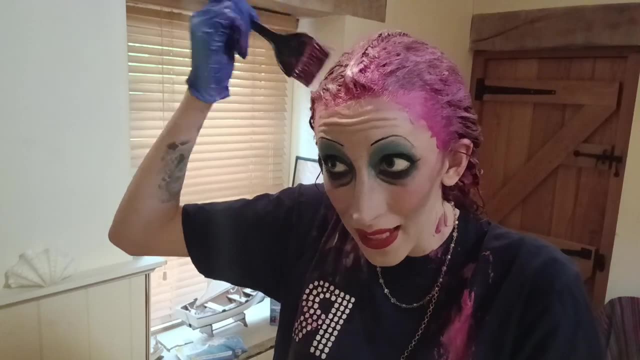 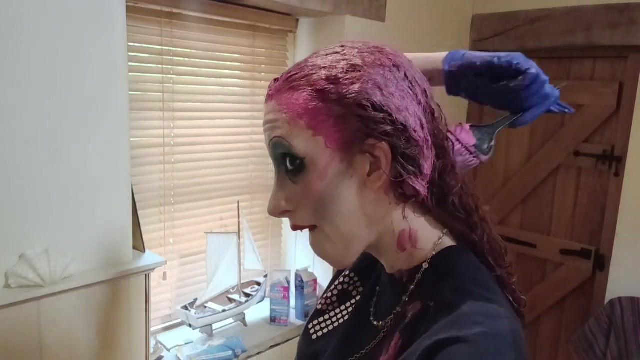 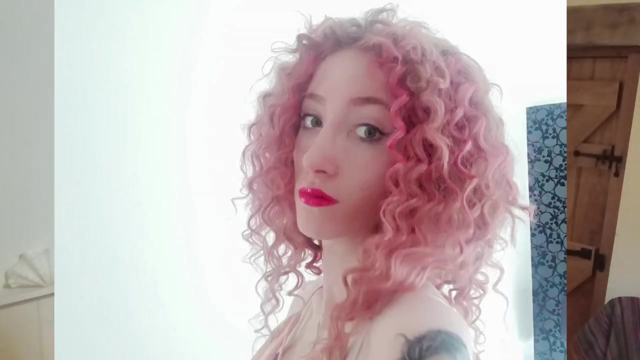 kind of shops. but um, the color. i'll insert a picture of this. the color wasn't actually that bright like it was a pretty faded, dull pink. and there's a picture i've still got on my instagram to this day actually, of me with this hair coloring, and i even edited that. i filtered the shit out of that picture and it's still um. 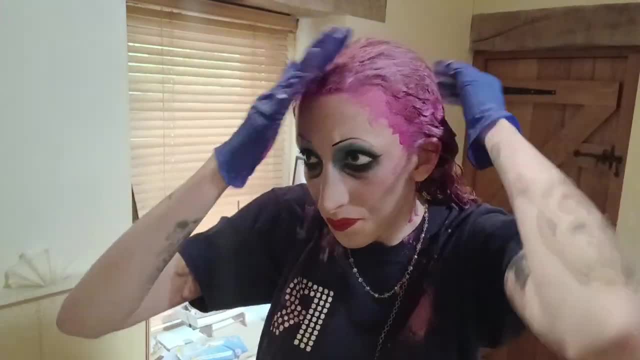 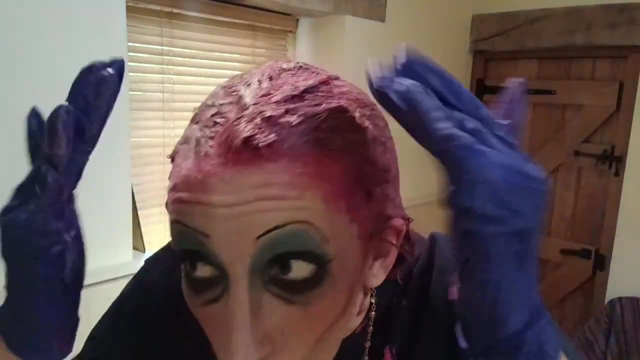 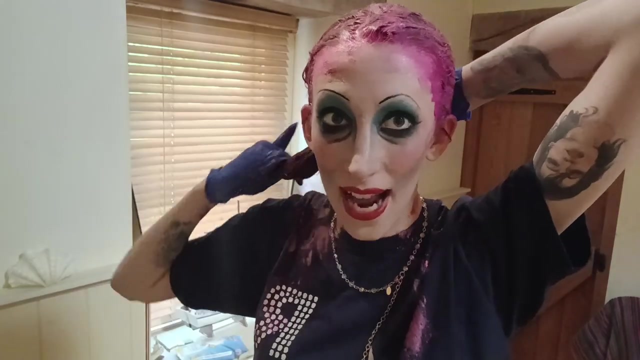 and the color is very fucking pale. so the next day i went back and i bought this exact stuff i'm putting on my head right now, and that got it to this color, which again i'm going to, which ideally is what i want today, and it's this very, very bright pink, and that was exactly what i wanted, like. it was like 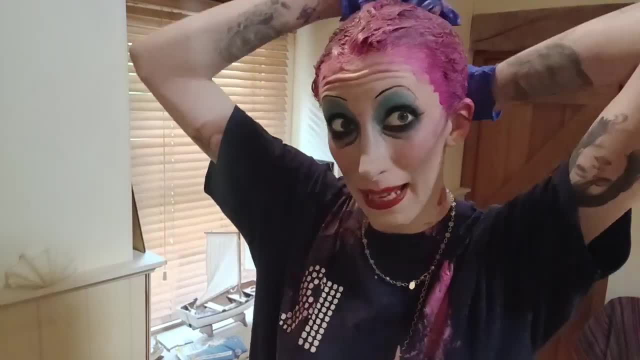 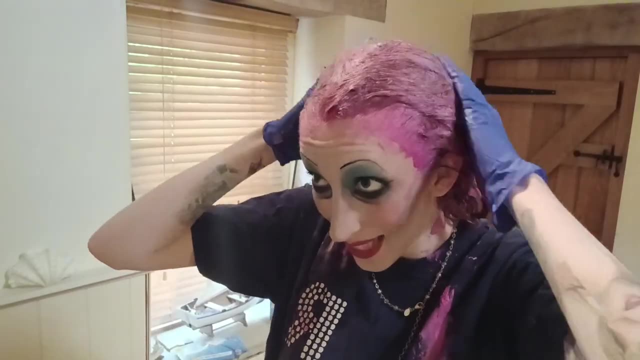 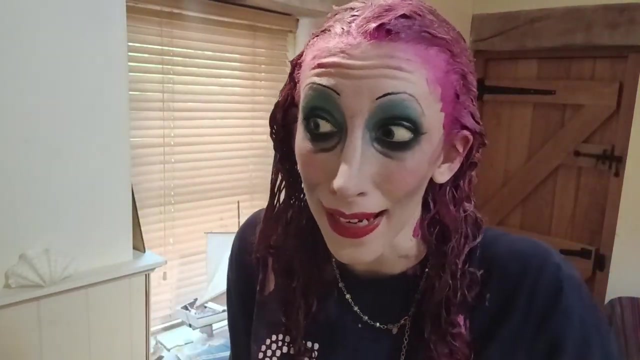 considering that i did put that over ginger, that went really, really pink. so that is um what i'm hoping for today, and i'm dying my hair in the exact same kind of conditions, i guess you could say, as i did back then. so theoretically that should be fine, i am. 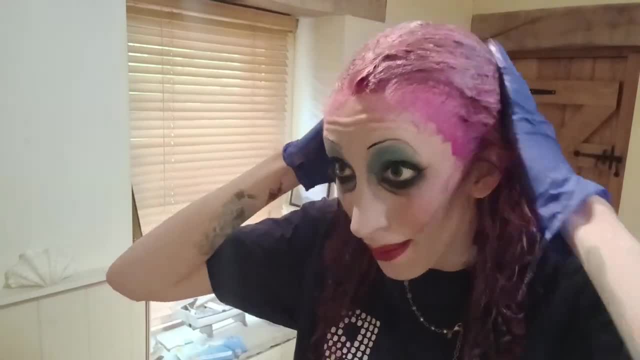 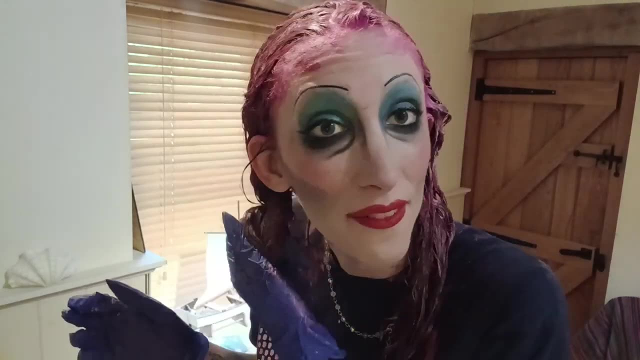 going to um, it's pretty much covered, but i can tell there's some areas that aren't really saturated as much as the rest and i do still have like a quarter of a bowl left down there. so, um, i'm going to do that, that off camera, so i don't have to think about you know. 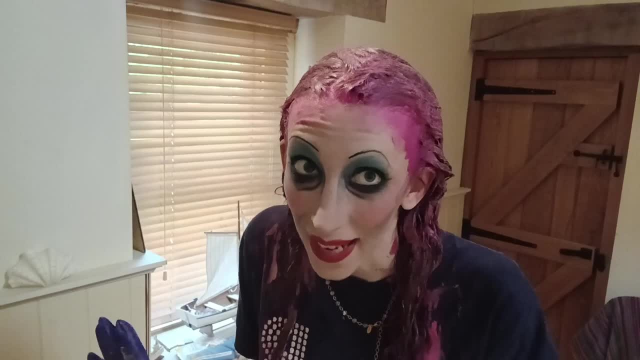 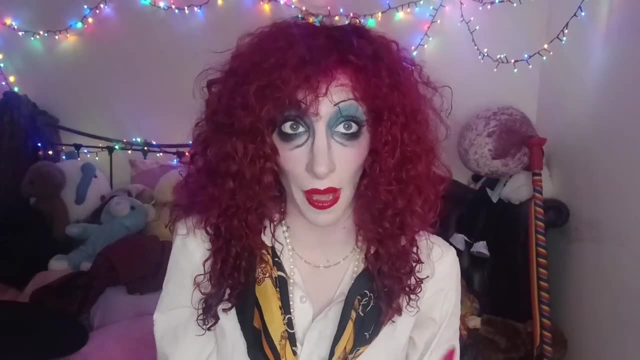 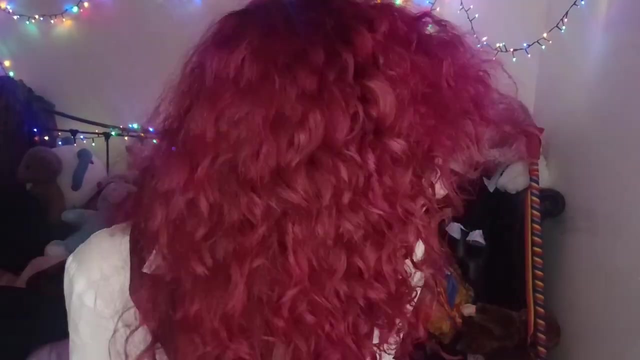 angles and shit gonna do that, and then I'm gonna wait and then we can rinse it off and do everything else. okay, so I am back, it is done, and I have several conclusions to draw about this. um number one at the minute. do I think this is worth it? no, because, um, this shit is not as pink as I expected. 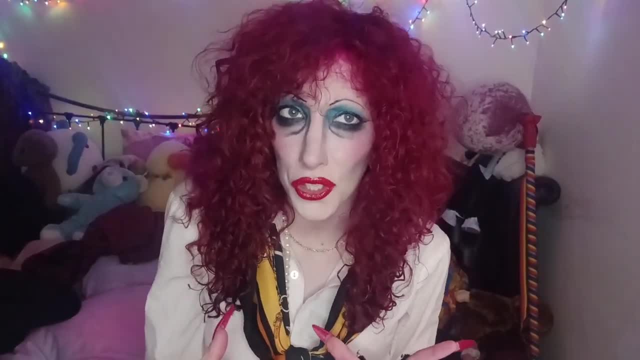 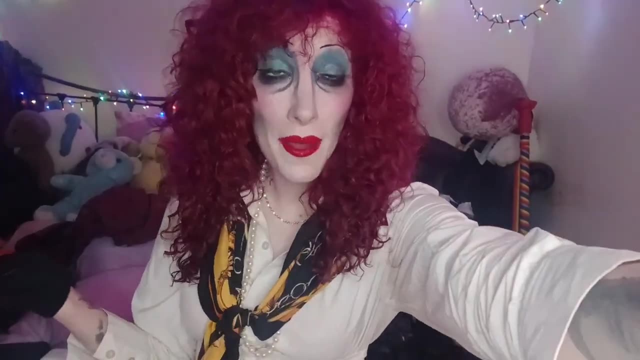 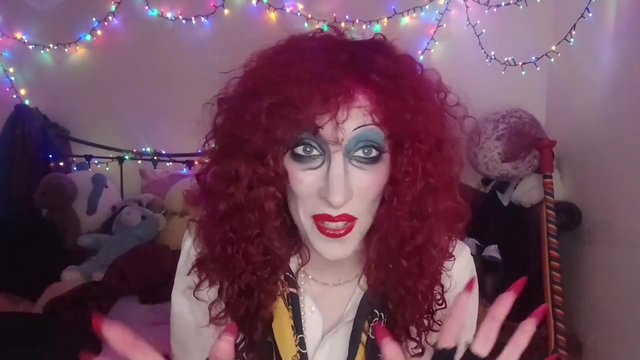 it to be like. to me this looks quite subtle, and if I dye my hair I don't want it to be subtle like. it still looks kind of gingery to me and, um, is that entirely my own fault for dying it over dark, ginger hair? yes, should I probably have left it on for longer and maybe use more boxes? yes, am I? 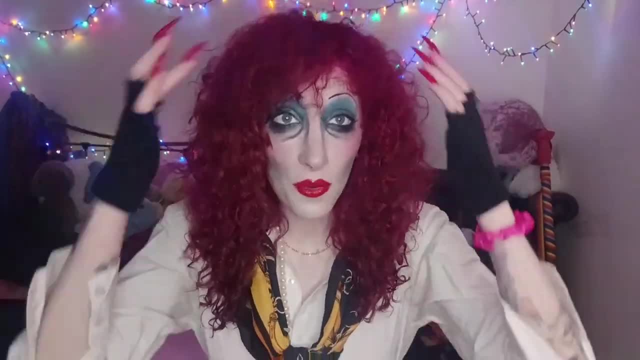 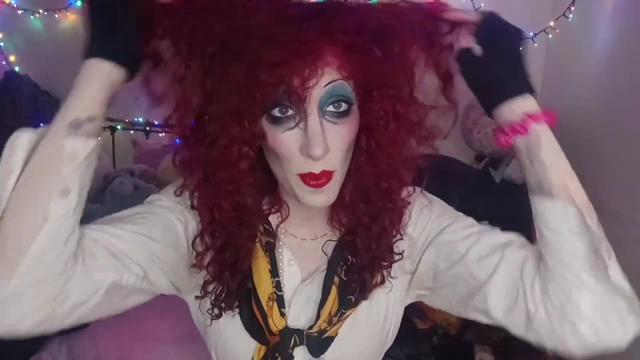 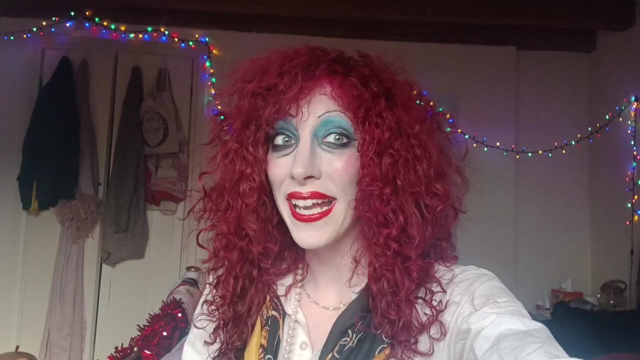 gonna do it again. no, so, um, I don't know how the lighting looks because, um, the window is there and I've just closed the? um blinds and put my ring light on, but I'm gonna try and shoot this in like an actual daylight and we'll see what the color looks like there. okay, there we go here. 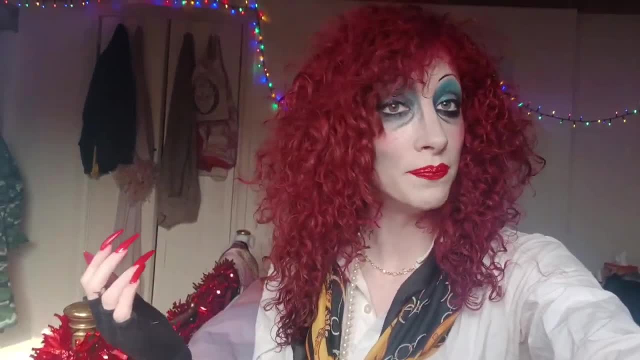 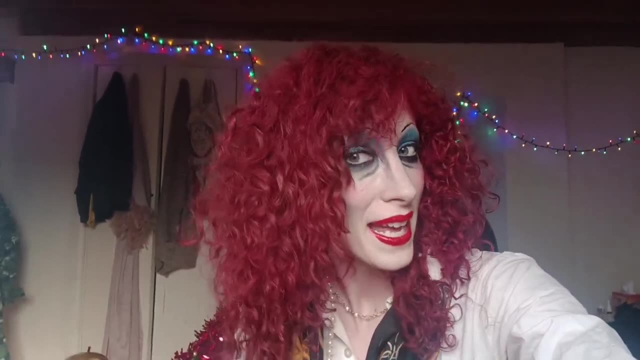 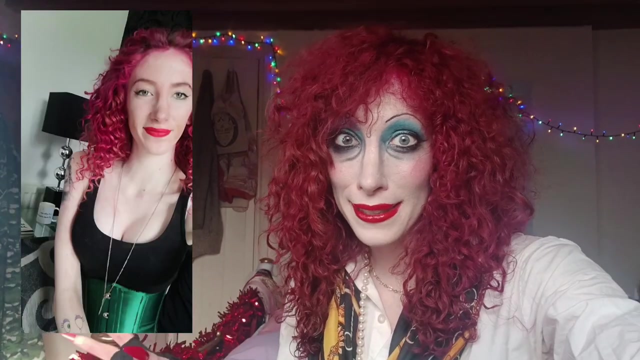 it is in more of a daylight because I'm in front of the window. um, yeah, so this is the color. it's not as bright as I wanted it to be. it's a very kind of muted pink. it seems quite understated to me like I was going for this, like when I last had pink hair. that was what happened and that was what I. 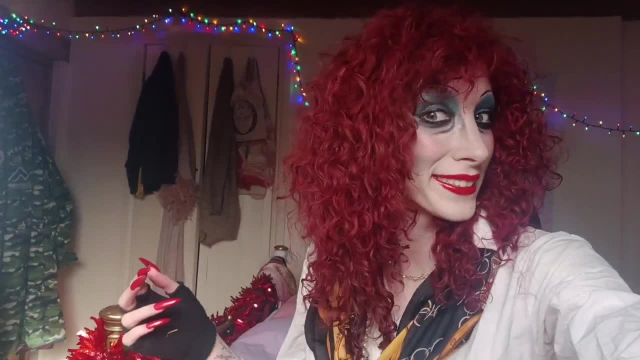 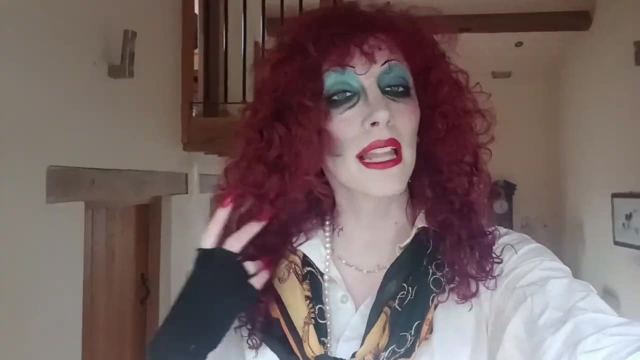 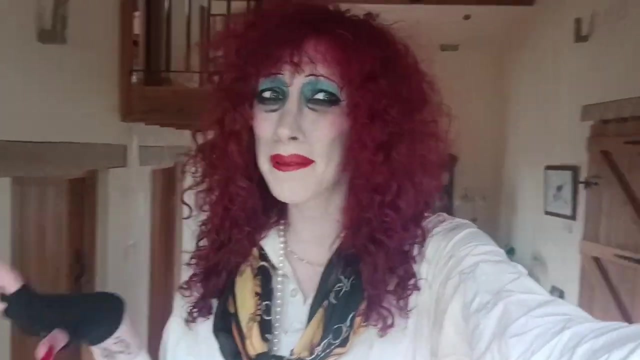 wanted, but um, evidently fate had different ideas. here we go. here's me in front of a big ass window and, um, I can't really tell in this camera lens, but um, yeah, this is essentially what I ended up with. is it gonna fade to ginger in a bit? probably, but I don't know. this is what happened. you're welcome. 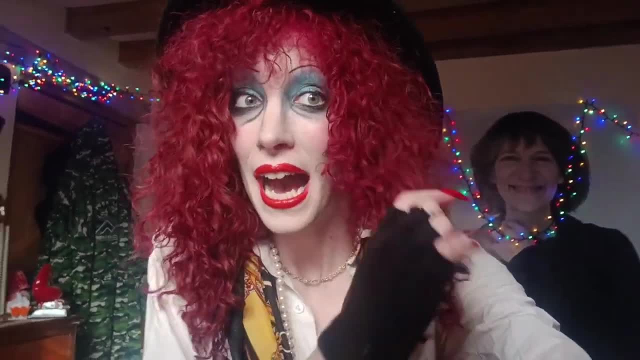 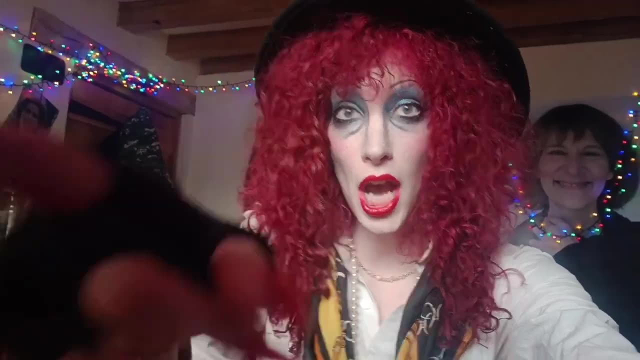 bye guys. let's watch that footage back. and I'm in that light. in whatever light I film this in, it just looks more red, like there's a mirror here. looking in this mirror: yes, it definitely does not look bright pink, but it still looks kind of pink.